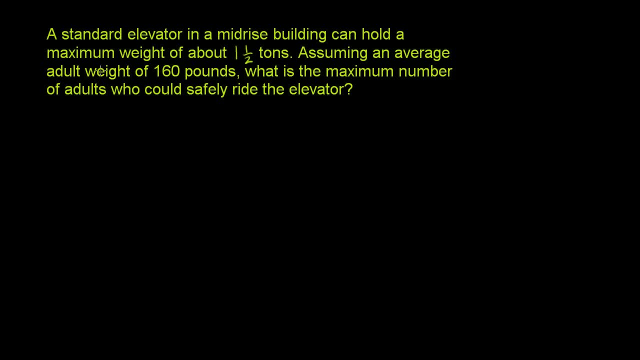 A standard elevator in a mid-rise building can hold a maximum weight of 1 and 1 1⁄2 tons, Assuming an average adult weight of 160 pounds, what is the maximum number of adults who could safely ride the elevator? So what we need to do is we have to get the maximum weight. 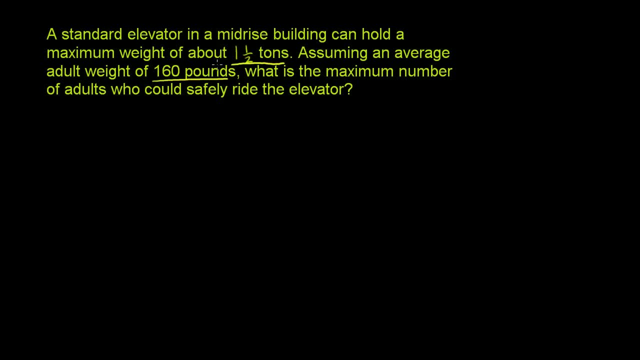 that the elevator can hold in terms of pounds and then just say, OK, well, how many adults is that? So they gave us the maximum weight in terms of tons. So they say it is 1 and 1 1⁄2 tons. 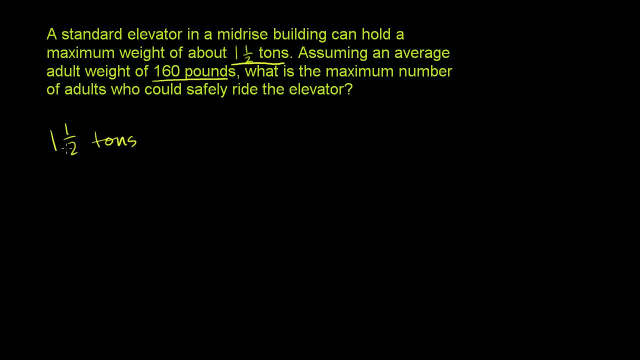 And it's always easier to deal with improper fractions than mixed numbers. So let's write this as an improper fraction. So 1 and 1 1⁄2 tons is the same thing as well. 1 ton is 2 halves, and then you add another 1 1⁄2, that's 3. 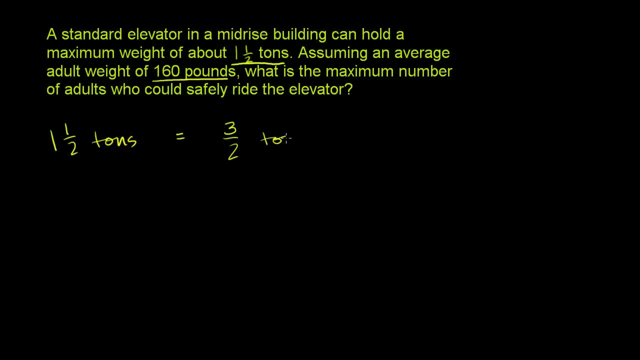 halves, so you get 3 1⁄2 tons. Or another way to think about it is: 2 times 1 is 2, plus 1 is 3.. So the maximum capacity is 3 1⁄2 tons. 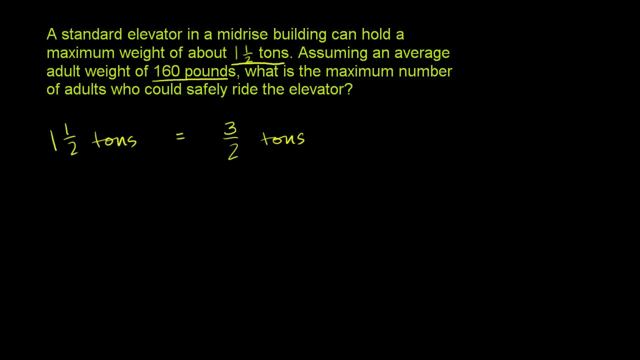 Let's think about it, How many pounds that is, And to do that we have to know that there are 2,000 pounds per ton. Let me write this up here: We know that there are 2,000 pounds per ton. 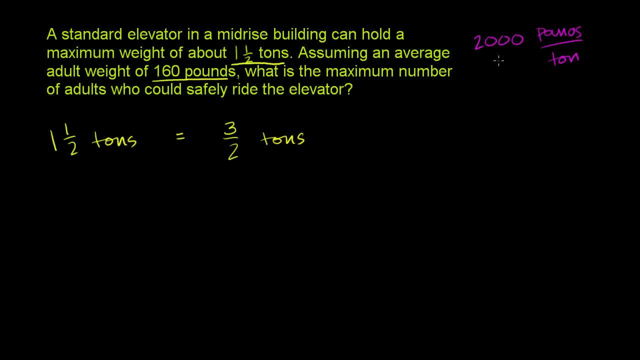 This wasn't given in the problem anywhere. This is something I knew from past experience. It's a good thing to know in general that a ton is 2,000 pounds, so I'm going to write it right over here Now: how do we convert these 3 1⁄2 tons into pounds? 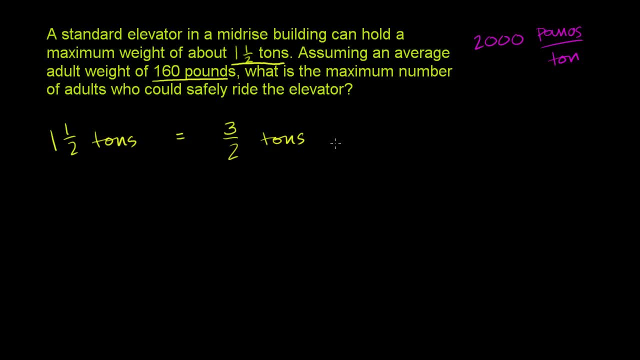 Well, we're going to multiply it by something And the units that we're going to multiply by. we want the tons to cancel out, So we're going to want to have tons in the denominator. We want tons in the denominator, so it cancels out. 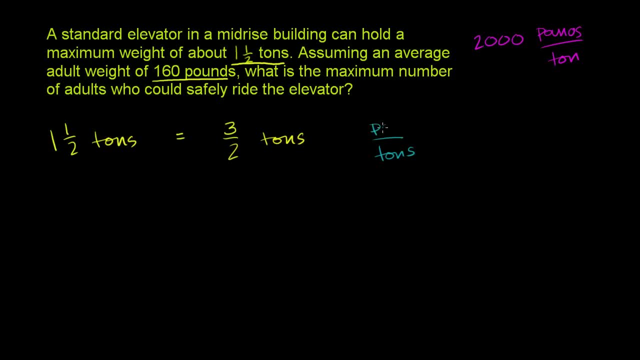 with this tons up here, And then we want pounds in the numerator And that's exactly what we wrote up here. There are 2,000 pounds for every 1 ton, or you could just say 2,000 pounds per ton. 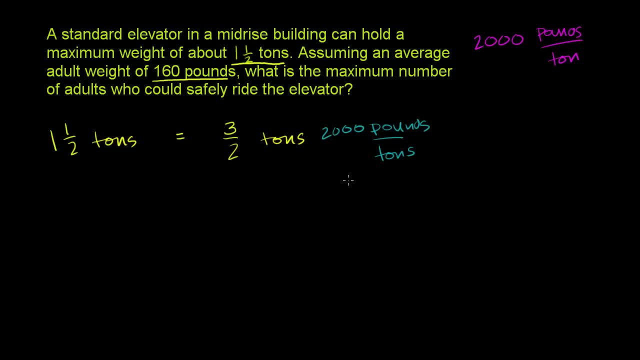 You could put the 1 there, but it doesn't really change the expression. Now, if we multiply 3 1⁄2 tons times 2,000 pounds per ton, what will happen is that the tons cancel out. That was the whole point of multiplying it by this. 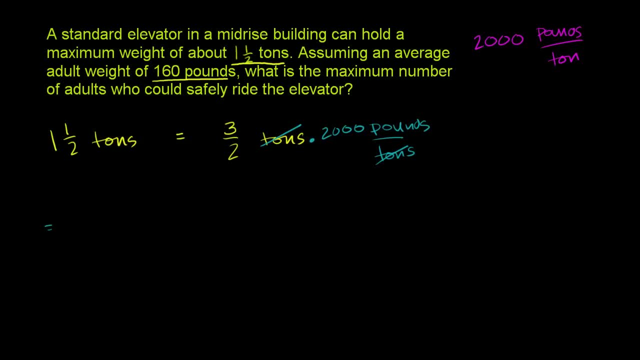 And we would be left with 3 1⁄2 times 2,000.. And the only unit left is pounds. If you do it this way, you'll never get confused. You'll know that the units cancel out. so you're getting. 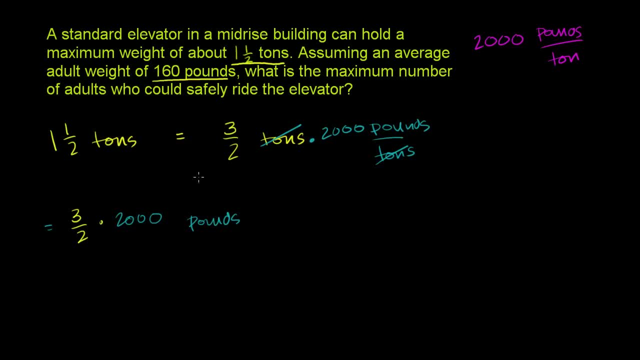 the right units. But if you just think about it in your mind, it should also make sense: If there are 2,000 pounds per ton and there are 1 1⁄2 tons, I should multiply 1 1⁄2 times 2,000 to get the number of. 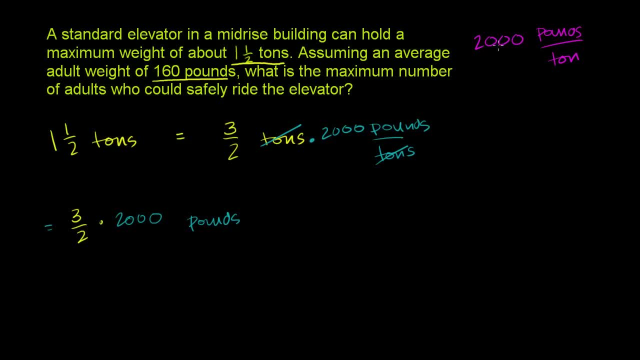 pounds. That makes sense. And we know 1 1⁄2 times 2,000 is 3,000, but we'll figure it out right here. So what is 3 1⁄2 times 2,000?? 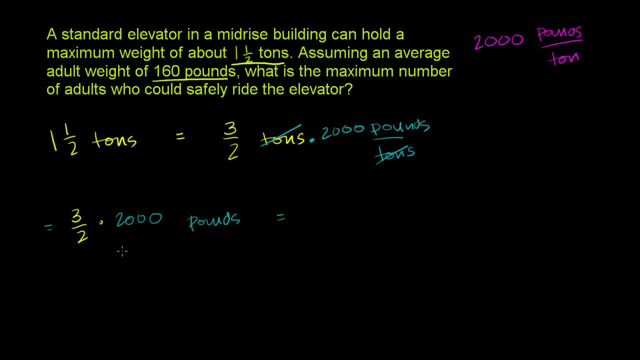 I just told you the answer. We can actually simplify it right over here. This is going to be 3 times 2,000 over 2 pounds. We can divide the numerator, We can divide the denominator by 2. This will become 1,000.. 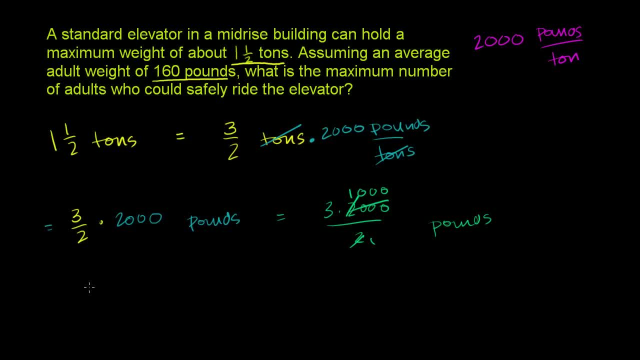 And this will become 1.. So it's 3 times 1,000 pounds, Or this is equal to 3,000 pounds. So what we've done so far, we've just figured out the maximum capacity of the elevator. It can hold 1 1⁄2 tons, which is the exact same. 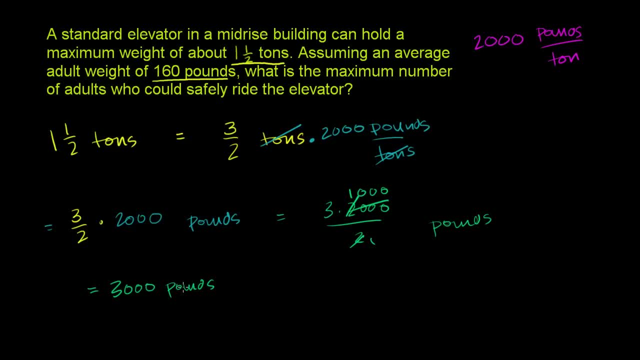 thing as 3,000 pounds. Now what we need to figure out is: 3,000 pounds is equivalent to how many average adults of 160 pounds, Or how many 160-pound people- 1 1⁄2? 1 1⁄2?? 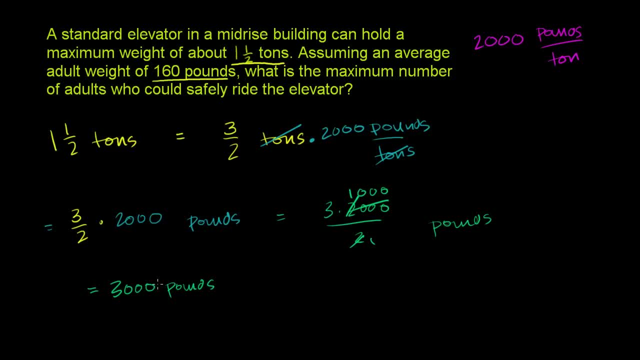 1 1⁄2 people, Would it take to weigh a total of 3,000 pounds? Well, we can just divide by 160.. And if you want to make sure that the units work out, remember we want our answer to be in terms of people. 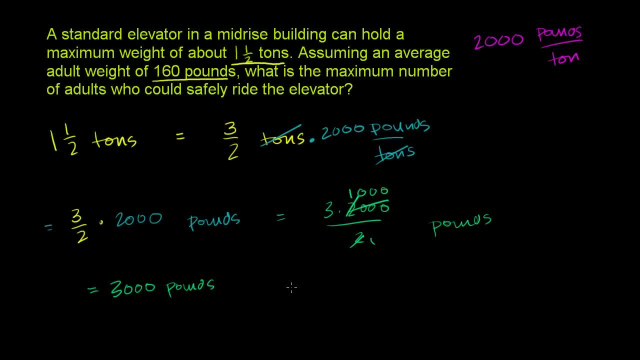 And we want the pounds to cancel out. So we have a pound in the numerator here, So if we divide by pounds, the pounds will cancel out. And then we want our left over to be people, or maybe person, Person, people- same thing. 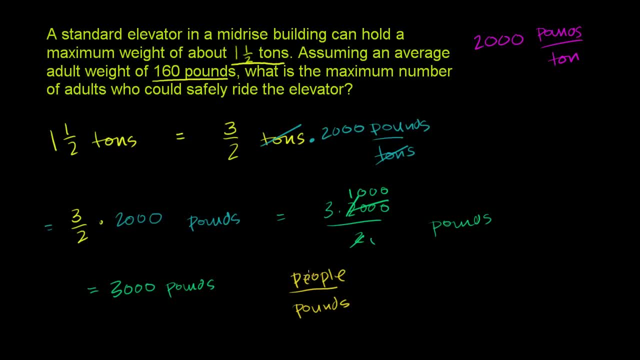 Let me do people. The grammar of it, or singular plural, might make it a little confusing, but I think you get the general idea. Now, if we were to write this out, what does it tell us? One person weighs 160 pounds. 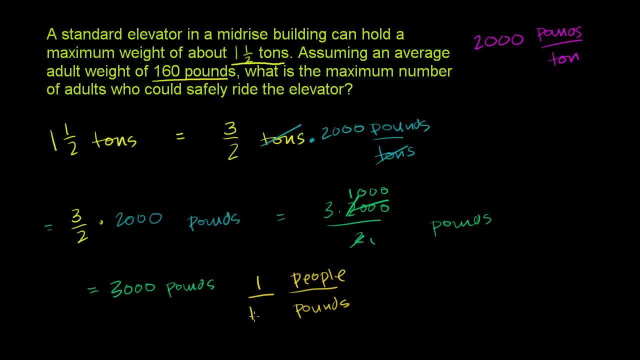 So there's one people or one person for every 160 pounds. So notice, if we multiply these two expressions, the pounds will cancel out. We'll be just left with people. But we're really just dividing. We're multiplying 3,000 times 1 over 160, but it's really just. 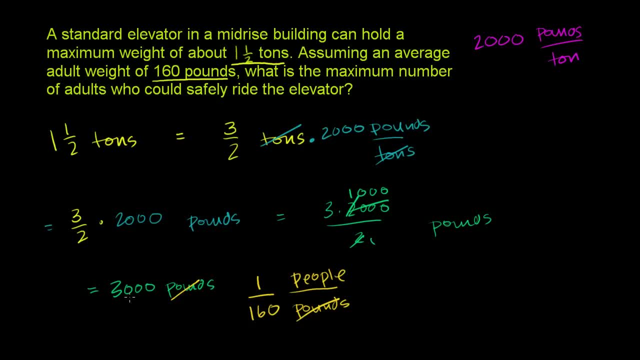 taking 3,000 pounds 3,000 and dividing by 160, which makes sense, We have a capacity of 3,000.. Each of our people weighs 160 pounds. Divide by 160 tells you how many people, But this way you know that the units are working out. 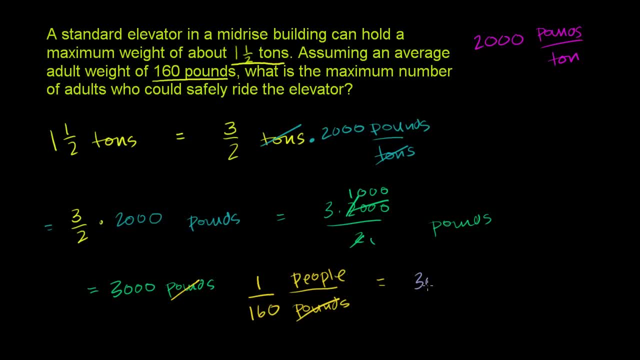 So this is going to be equal to 3,000 over 160 people. That is the maximum capacity of the elevator in terms of average people. Now, what is this? Well, we can divide the numerator and the denominator by 10.. 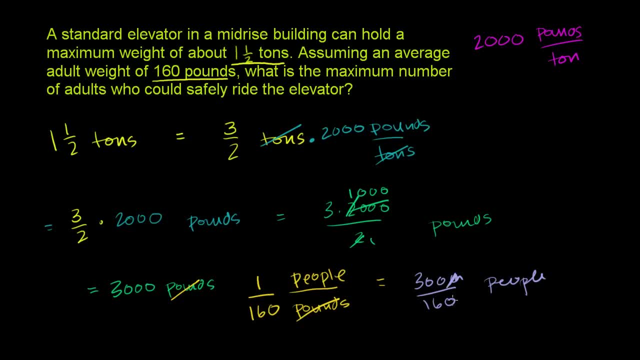 If we divide the numerator and the denominator, we get 150.. If we divide the denominator by 10, this becomes 300 over 16.. If we divide 300 by 2, this becomes 150.. If we divide 16 by 2, this becomes 8.. 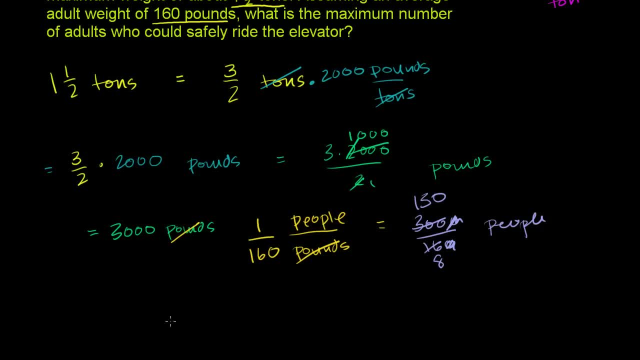 Now let's see What can we do more here. Well, we could divide by 2. again, Let me rewrite it. So this is the same thing as 150 over 8 people. See 150, we can divide by 2.. 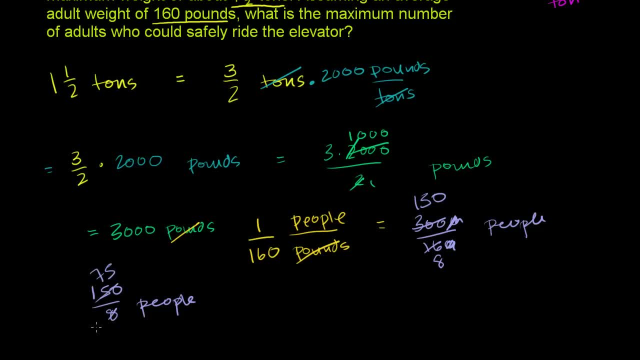 This gives us 75.. And if you take 8 divided by 2, that's just going to give us That is 4.. So we have 75 divided by 4 people. Let me just do that work it out. So you have 75 divided by 4.. 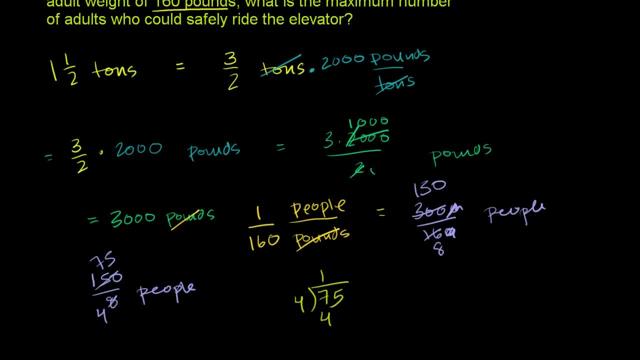 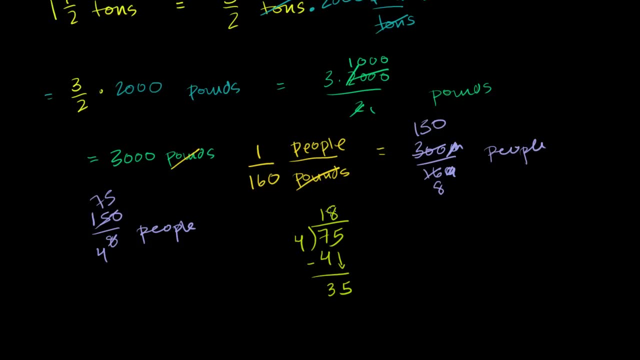 4 goes into 7 one time. 1 times 4 is 4.. You subtract 7 minus 4 is 3.. Bring down this: 5.. 4 goes into 35. 8 times. 8 times 4 is 32.. 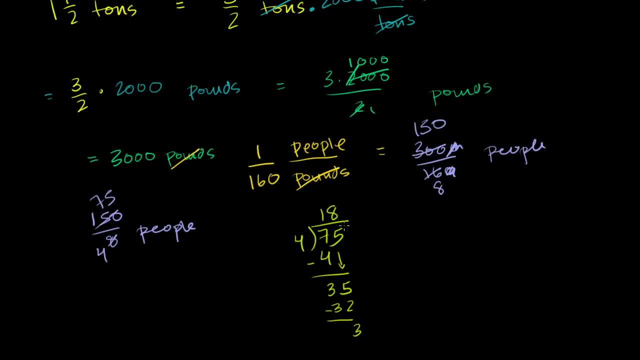 Subtract 5 minus 2 is 3.. And then you have the decimal. We're going to the right of the ones place. We're going to the tenths place now, So we can bring down a 0 over here. 4 goes into 30, 7 times.